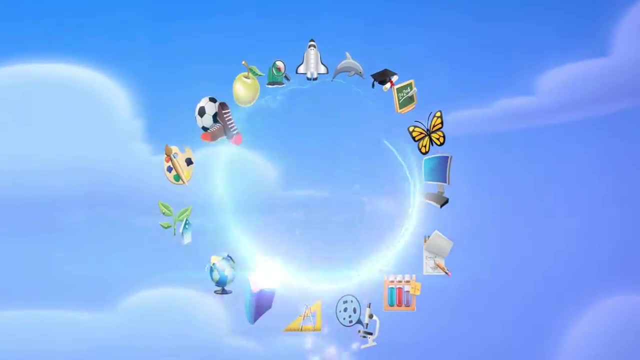 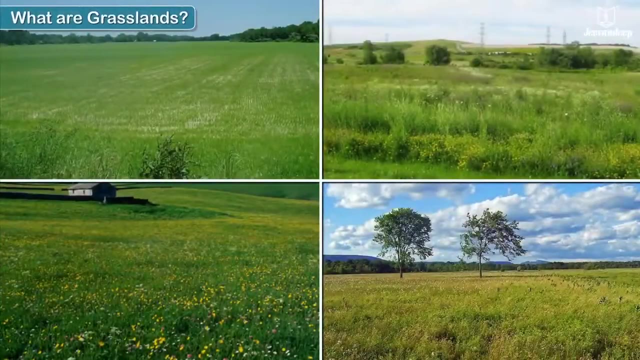 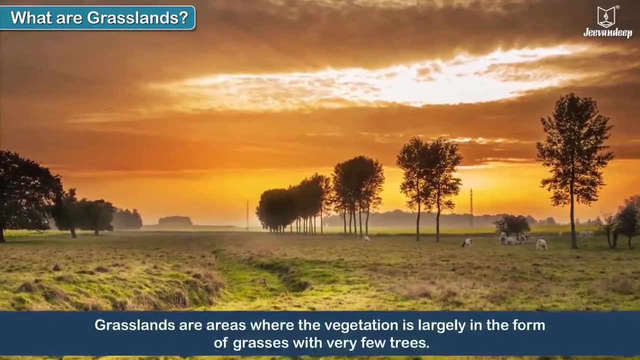 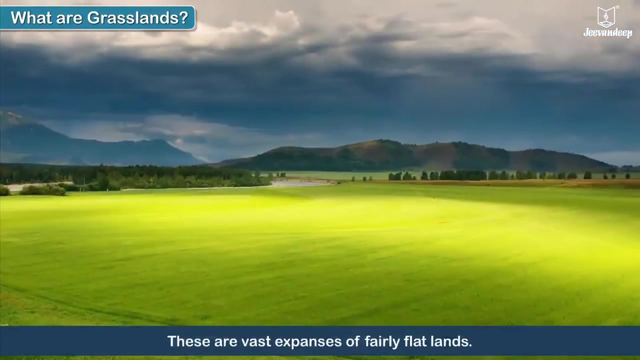 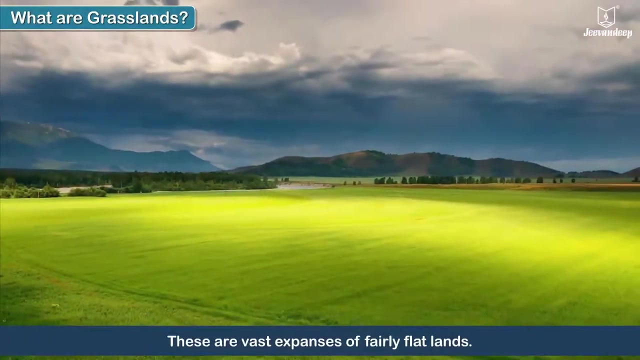 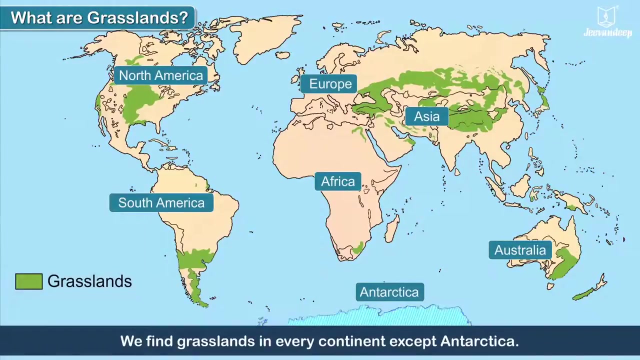 What are grasslands? Grasslands are areas where the vegetation is largely in the form of grasses, with very few trees. These are vast expanses of fairly flat lands. We find grasslands in every continent except Antarctica. Most of these areas are present in the drier interiors of the continent. 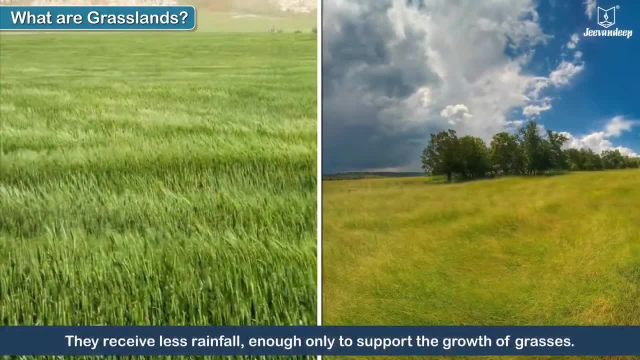 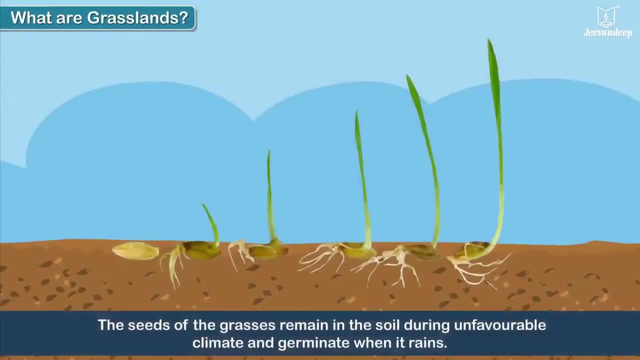 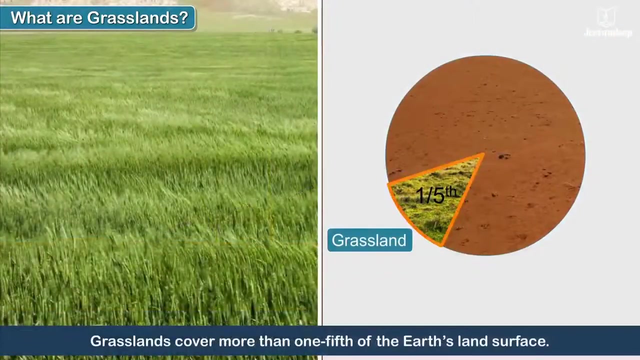 They receive less rainfall enough only to support the growth of grasses. The same is true for the grasslands. Seeds of the grasses remain in the soil during unfavorable climate and germinate when it rains. Grasslands cover more than one-fifth of the Earth's land surface. 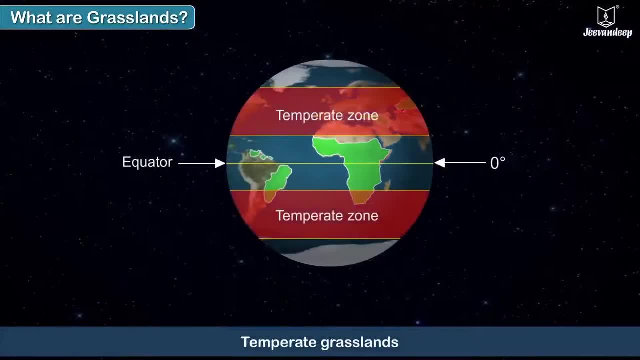 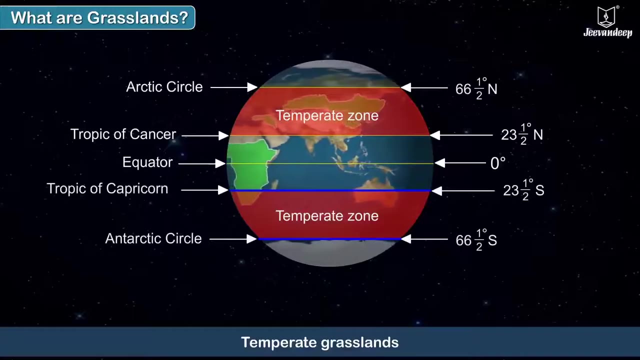 The temperate grasslands lie in the temperate zone Between latitudes 23.5°N and 66.5°C. the temperate grasslands live in valleys around an altitude of 65°uesto and 64.5°S in a city per một meter above groundLER Fallout. 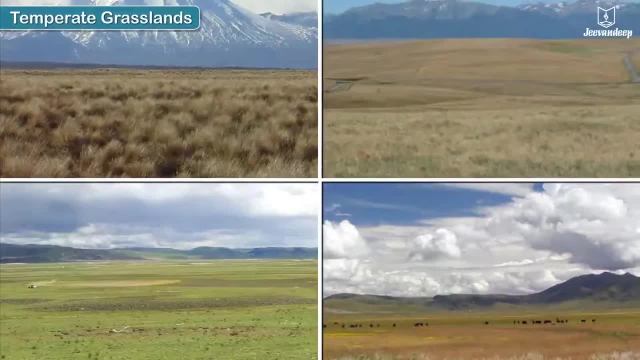 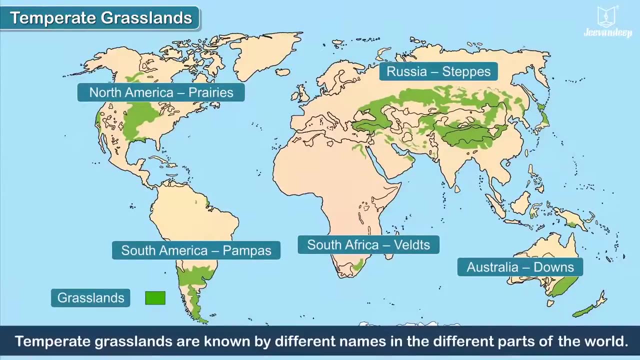 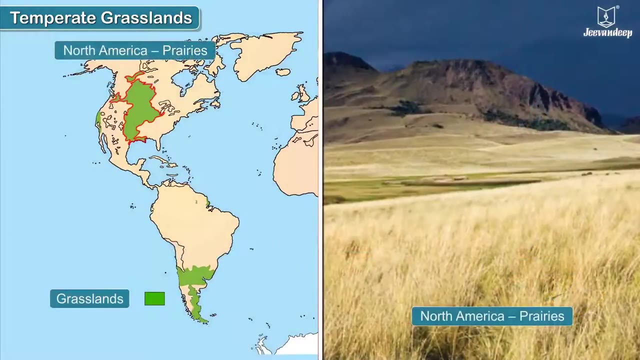 Temperate grasslands. Temperate grasslands are known by different names in the different parts of the world. In North America, they are called prairie stakes, while they are known as pampers. While they are known as pampers because they are crushed trees. they are therefore called prairie stakes and are satisfrical growers of洲. While they are known as pampers, they are also known as scultures. While they are known as pampers, they are still sometimes called god-forsaken villages. While they are known as pampers, they are sometimes called prairie ERIC, etc. which are said to eliminate the problem of history of prairie trees. 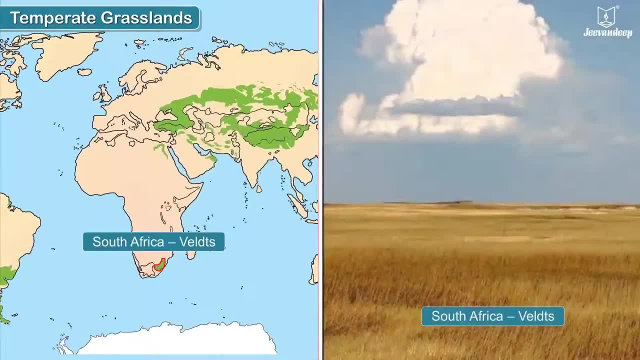 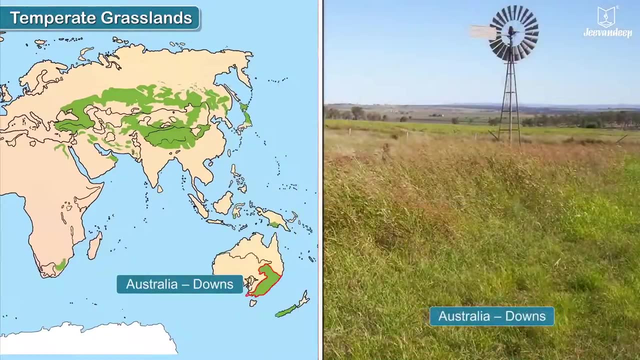 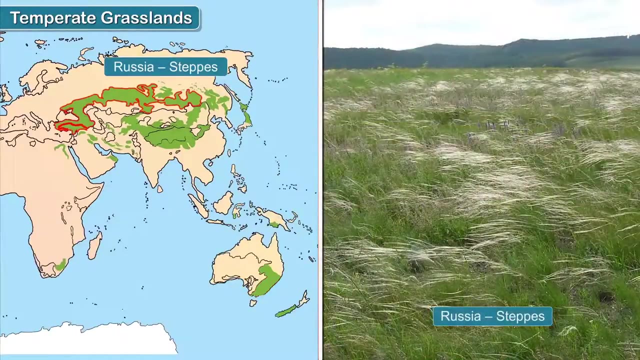 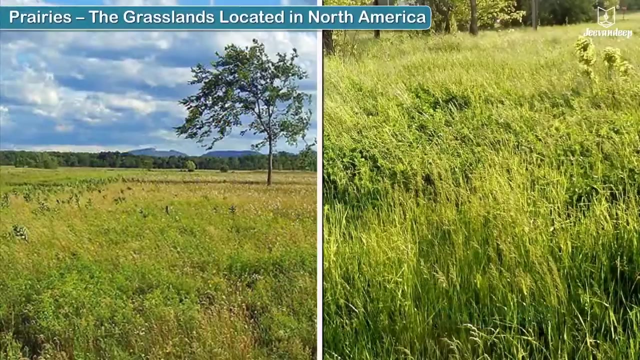 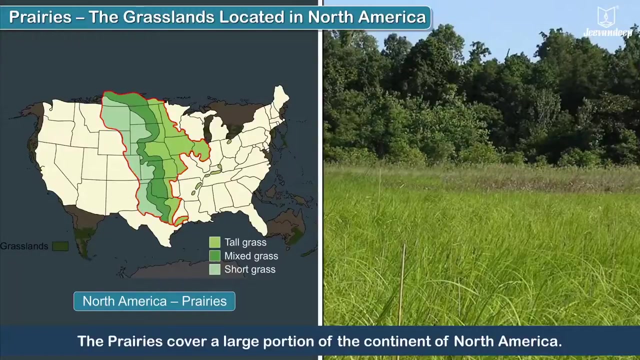 South America. In South Africa, grasslands are known as wells, In Australia they are called downs and in Russia they are known as steps Prairie grasslands located in North America. The prairies cover a large portion of the continent of North America, stretching from the central part of the United States of 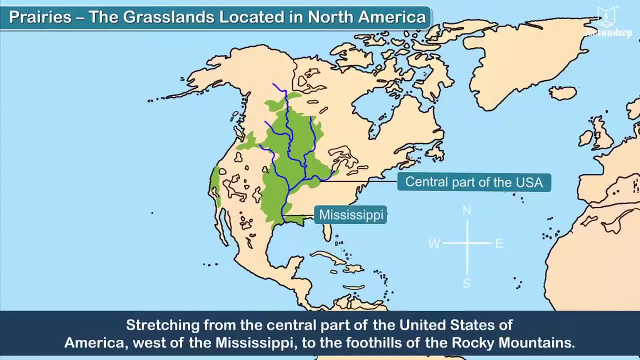 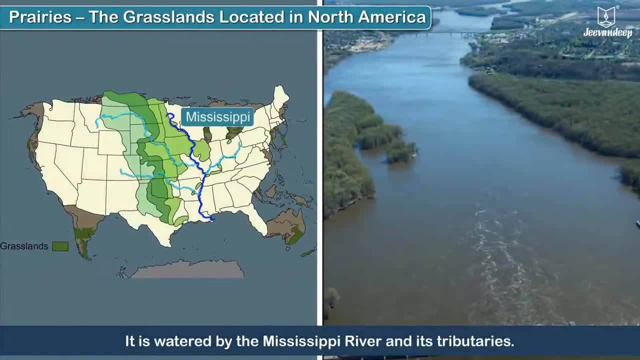 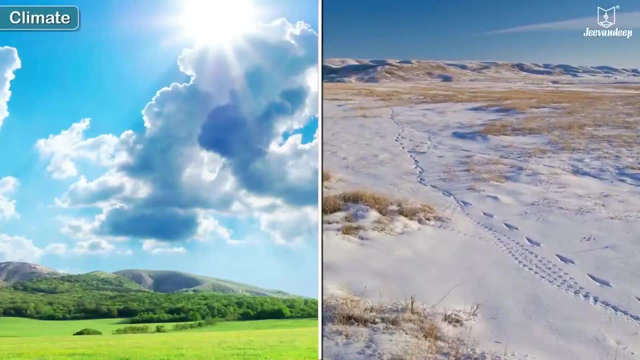 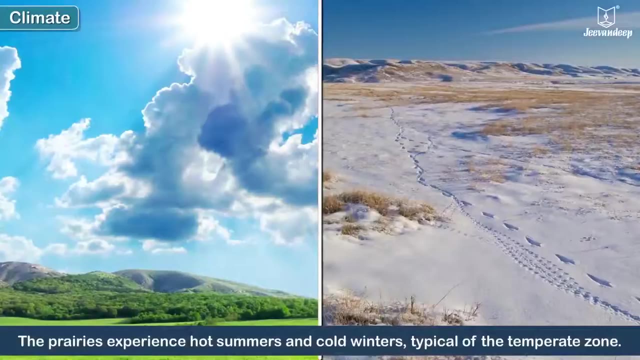 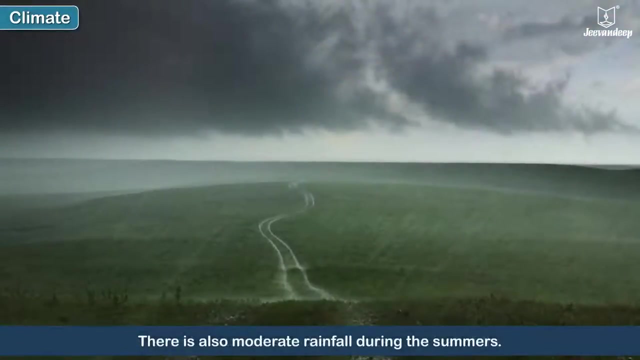 America, west of the Mississippi to the foothills of the Rocky Mountains. It is watered by the Mississippi River and its tributaries. Climate: The Prairie experience hot summers and cold winters, typical of the temperate zone. There is also moderate rainfall during the summers. Winters are 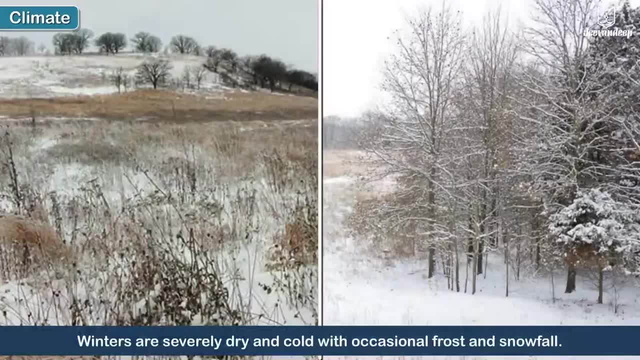 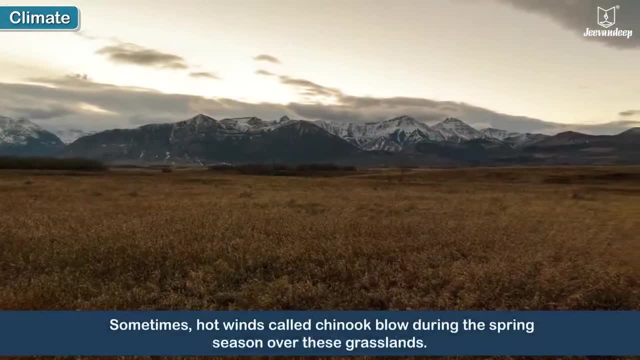 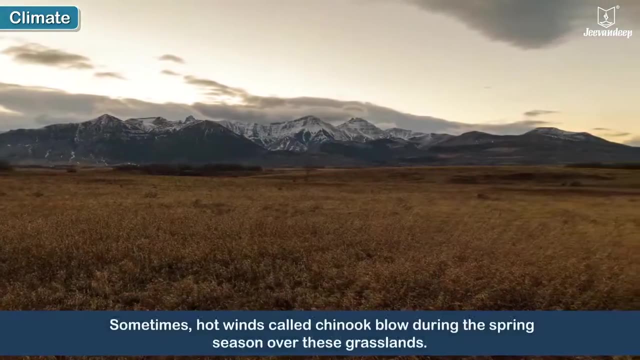 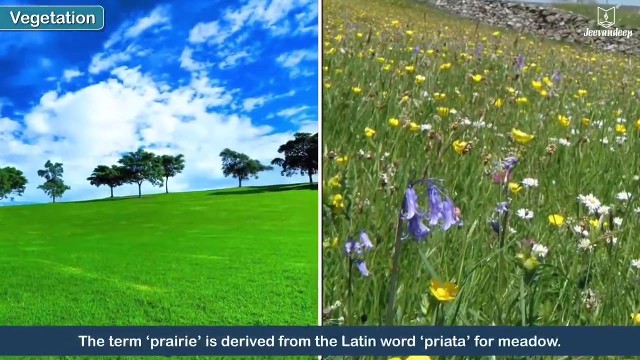 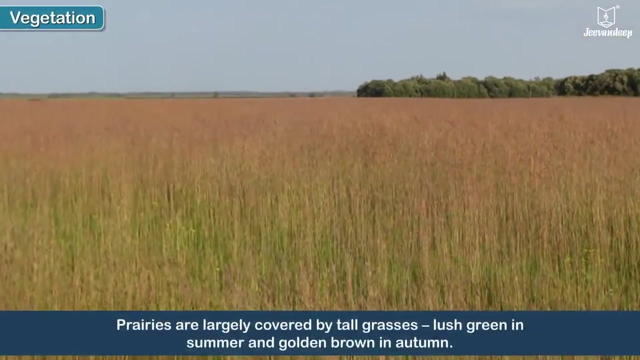 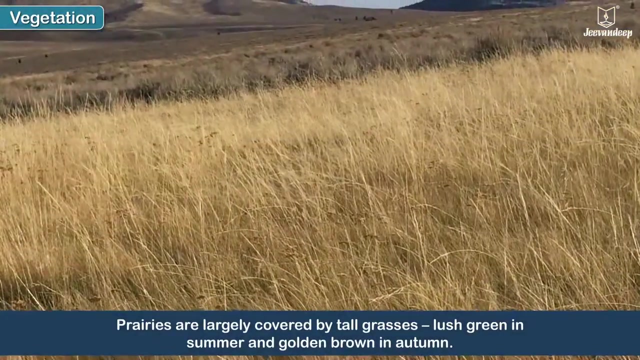 severely dry and cold, with occasional frost and snowfall. Sometimes hot winds, called chinook, blow during the spring season over these grasslands Vegetation. The term prairie is derived from the Latin word praetor for meadow. The prairies are largely covered by tall grasses, lush green in summer and golden brown in autumn. 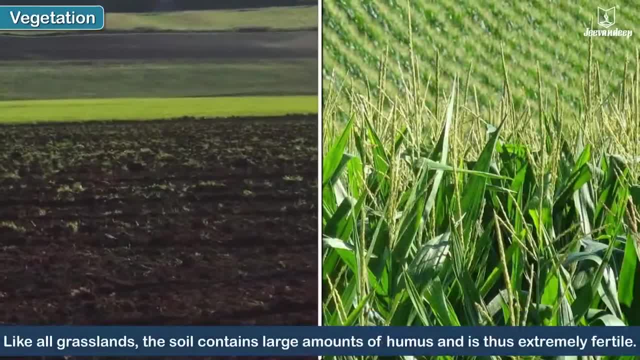 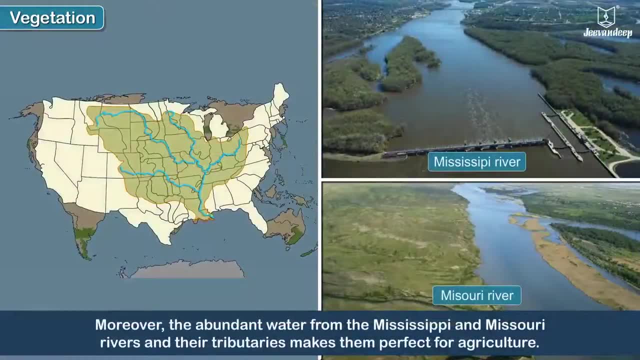 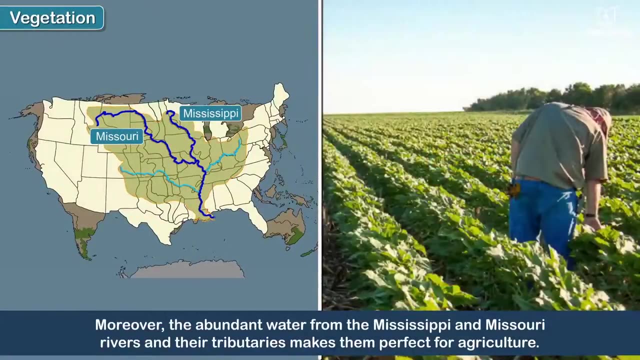 Like all grasslands, the soil contains large amounts of humus and is thus extremely fertile. Moreover, the abundant water from the Mississippi and Missouri rivers and their tributaries makes them perfect for the summer season. The prairie is also known as the prairie of the prairie. 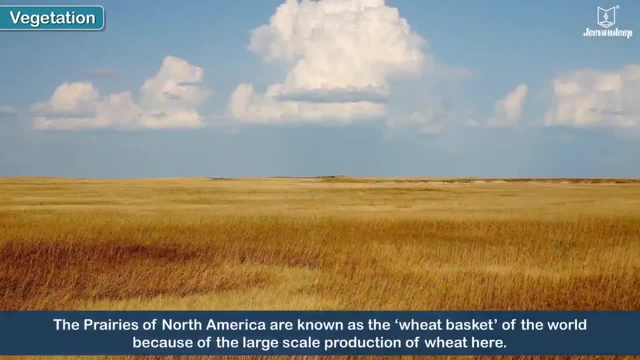 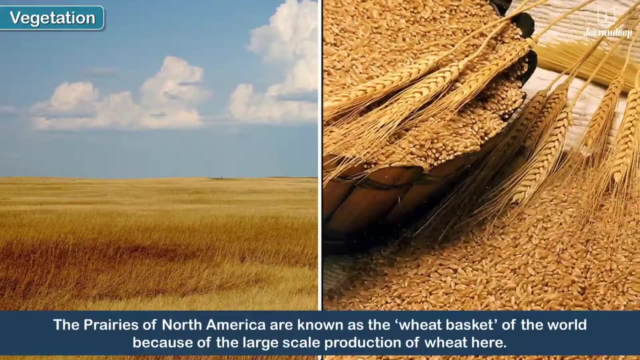 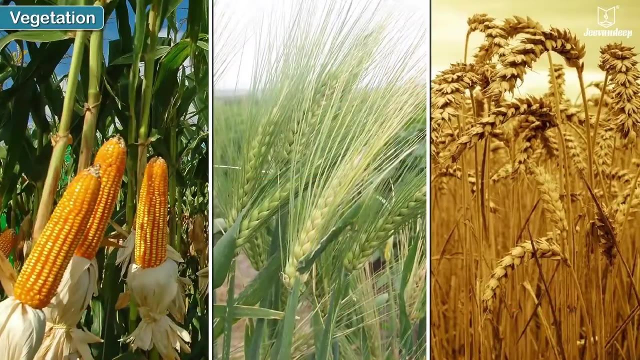 The prairie is also known as the prairie of the prairie. The prairies of North America are known as the wheat basket of the world because of the large-scale production of wheat here. The other crops grown here include maize, barley and rye. 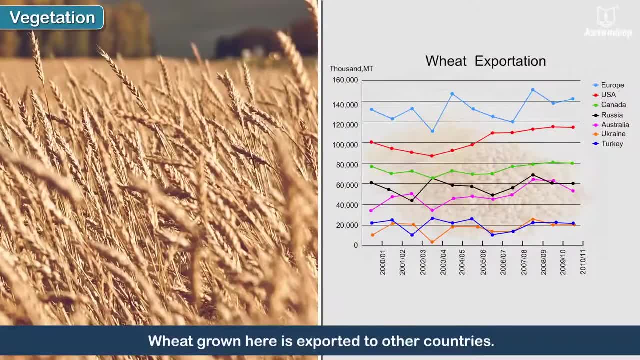 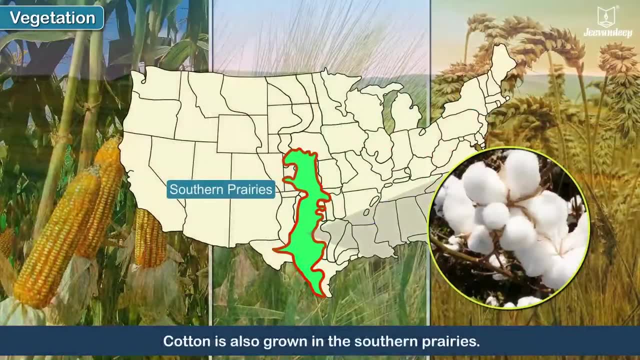 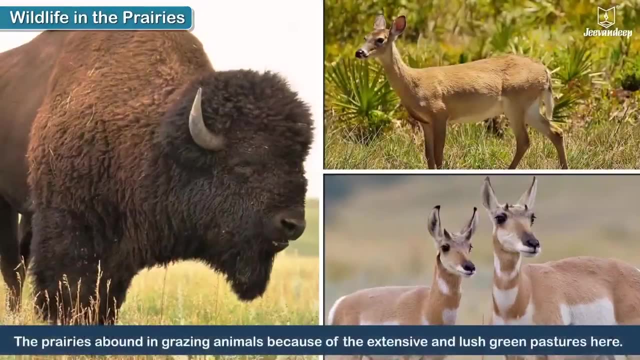 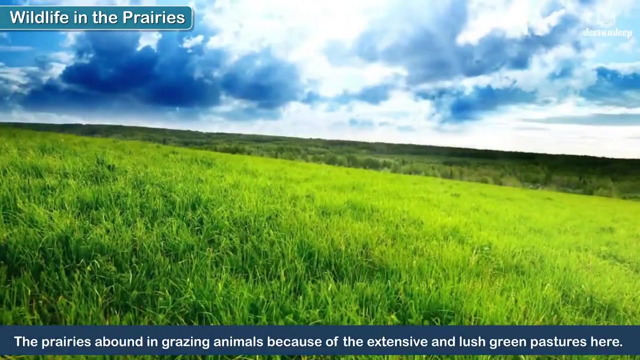 Wheat grown here is exported to other countries. Cotton is also grown in the southern prairies. Wildlife in the prairies abound in grazing animals like the bison, deer, pronghorn, etc. because of the extensive and lush green pastures here.